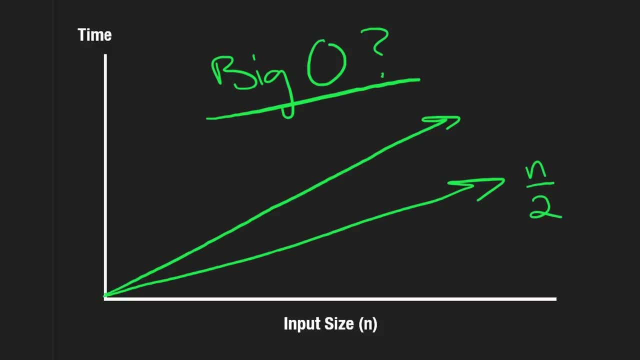 You could have another function like this, which is, for example, N divided by two, but we actually don't care about the differences, when those differences our constant values. we only care about the variable here, which is N. We don't care about. 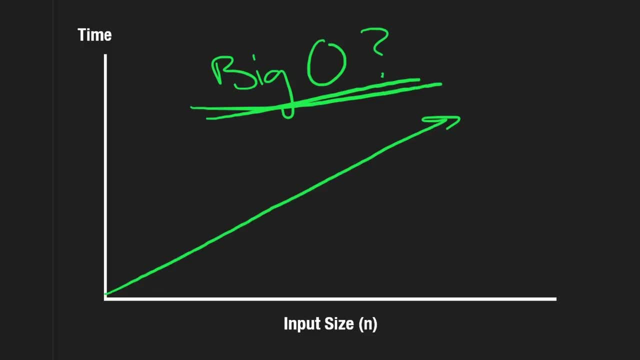 the divided by two, And that's true for all big O runtimes. We also don't care. if you know, we have N plus some constant like five, like that might look something like this on our chart: It just starts at a different spot and has the same exact slope. but we don't care about these. 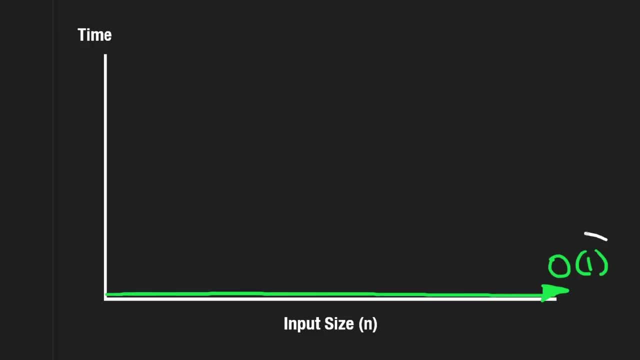 constants either. So the first runtime we're going to look at is big O of one. I know we said that we don't care about constants, but in this case, special constant that we do care about And, as you can tell from the chart, no matter how much. 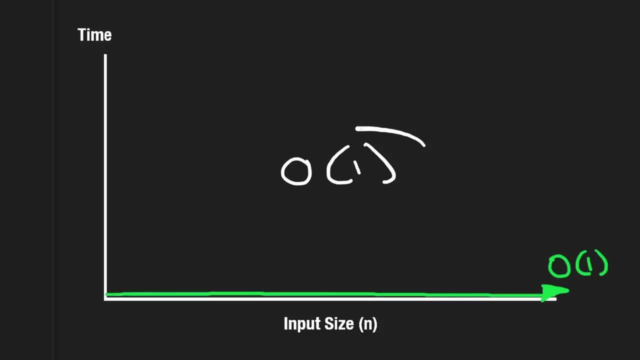 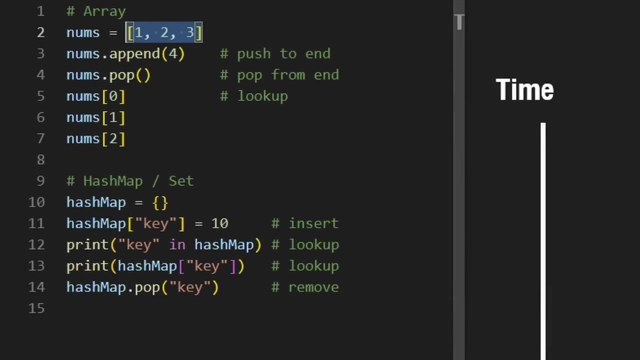 our input size grows the time complexity of big O of one time algorithms is always the same. You can see it's a flat line because the time it takes for these algorithms does not change based on the input size. These are the most efficient algorithms. So, for example, if you have an array of values, 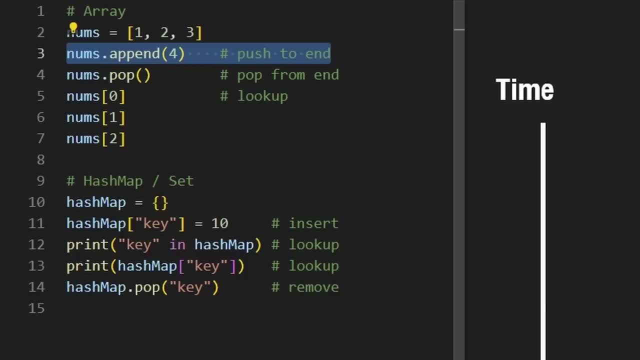 like this. it's a constant time operation to add to the end. It's also a constant time operation to remove from the end, or just to search an arbitrary index, just to look up a value at any index, whether it's at zero or one or two, And the same is true typically for a hash map. So to insert. 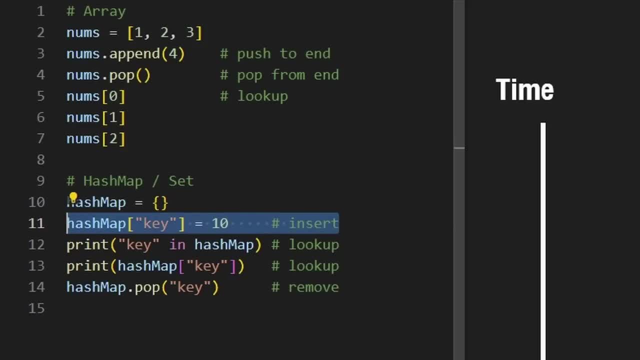 any value into a hash map is constant time. to look up a key from a hash map is also constant time, And to remove a key from a hash map is also a constant time operation, And the same operations could be applied to hash sets as well. We also have big O of N plus one, So we don't care about. 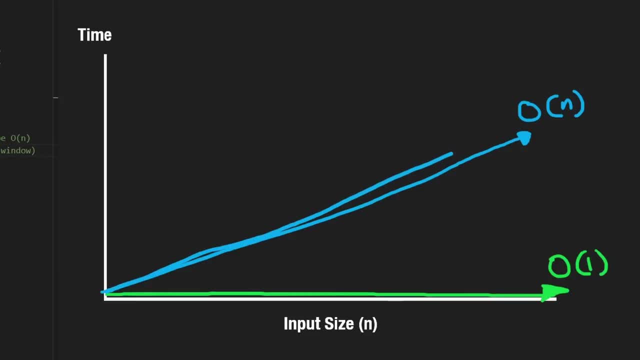 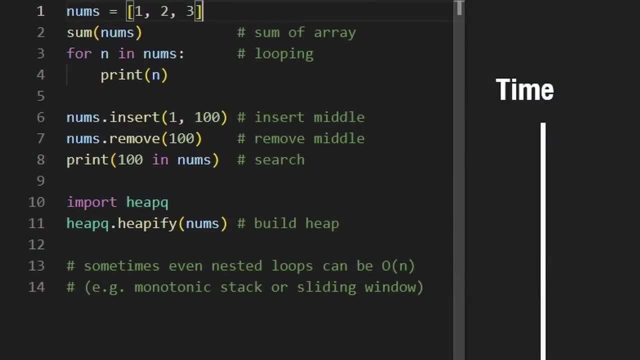 the value of n which, as we discussed, is the linear growth scenario. So as our input size grows, our time is going to grow proportionately. So if we're given some array of values and we want to take the sum of all of those values, this sum function is going to be a linear time algorithm. 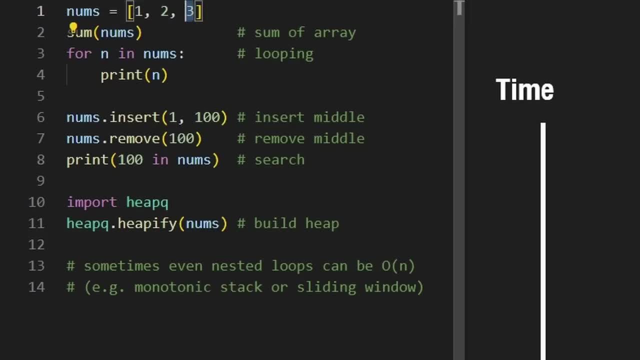 because we're going to have to go through every single number in the array. So with just three values it won't be too bad. But as our input size grows, so if our array had a million values in it, so then the runtime of calculating the sum would also grow, And of 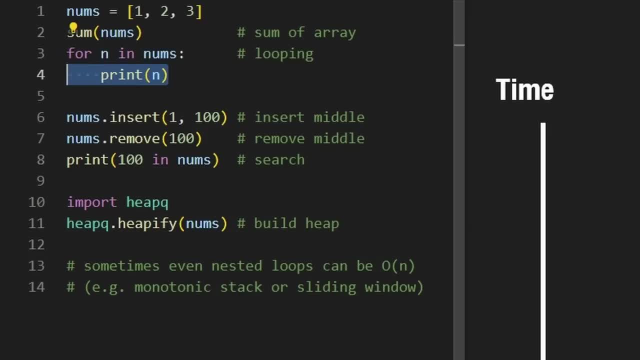 course we know that's going to happen because under the hood we're going to have to loop through all of the elements. So looping through a list of elements is also a linear time algorithm. inserting in the middle of an array and removing from the middle of an array is also big O of n. 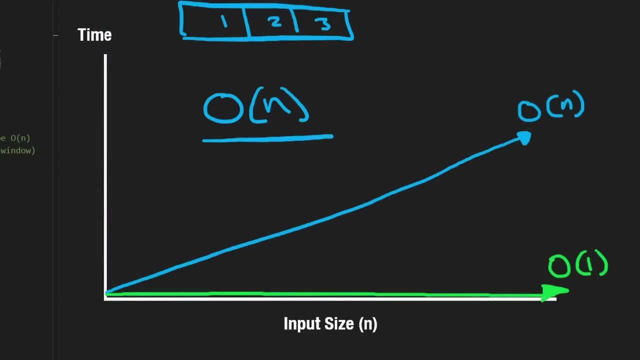 And that's because when we talk about big O of n, we mean the worst case, runtime, because in some cases, like inserting in the middle- well, for example, inserting in the middle of this array could be over here, in which case we would have to, you know, put a value. 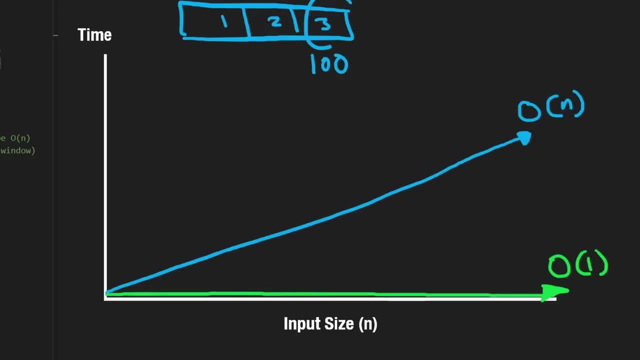 let's say we're inserting the value 100, we'd put 100 over here and then move the three into the next position, And then this would be our new array. So in this case we only had to move a single value. But what about if we wanted to insert the hundred over here? then we would have. 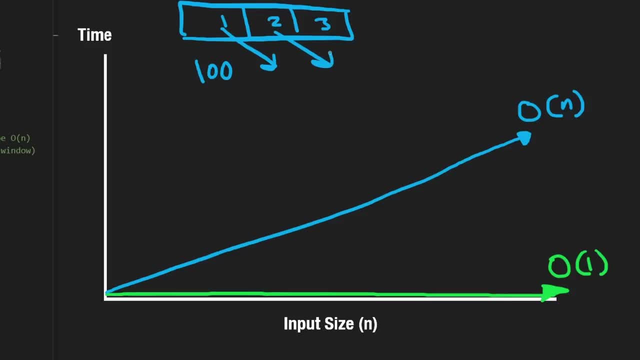 to insert the hundred here, we'd have to move the one to the right, we have to move the two to the right and we'd have to move the three to the right, so that this would be our new array, And in this example we had to move every single value in the array. we know that's an. 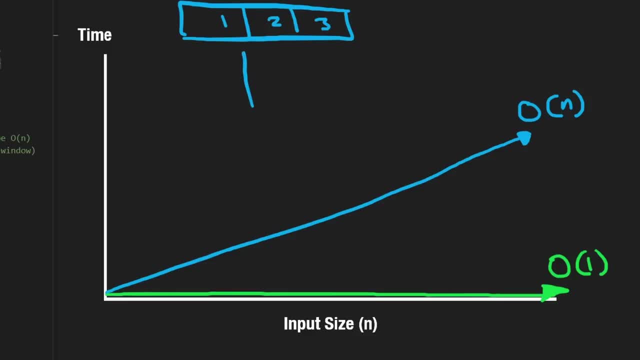 end time operation. So since we don't know where we might insert in the middle, we take the worst possible case, which would be big O of n. in this case also, removing from the middle is going to be similar. if we remove from the end, it's a constant time operation. But if we move from, 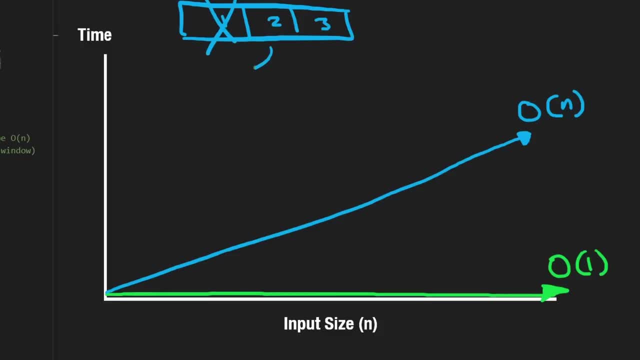 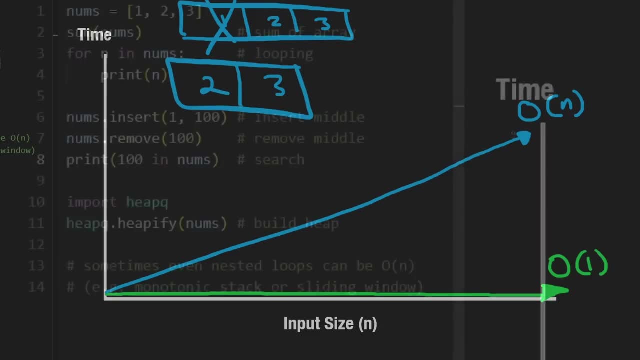 an arbitrary position, for example the first position, then we would have to shift every other value to the left and we'd end up with an array that looks like this: Now, searching an array is also a linear time algorithm. In the worst case, we would have to: 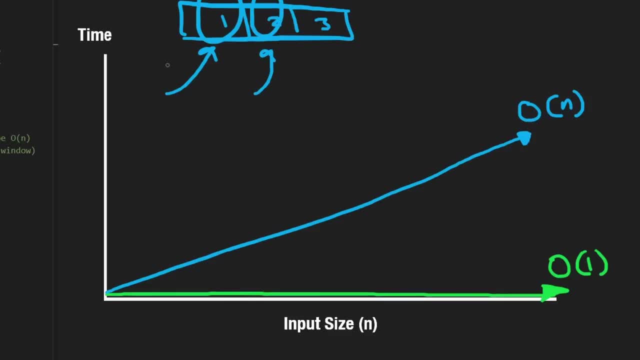 look at every single element in the array before we realize that the element- in this case if we're looking for 100- doesn't exist. it didn't exist anywhere And we had to look through the entire array to figure that out. Or we might find the element. we might even find it in the first. 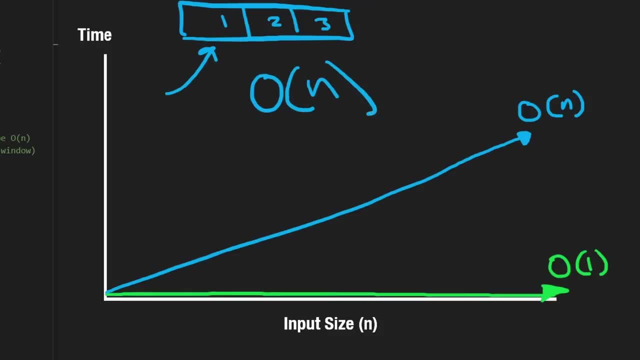 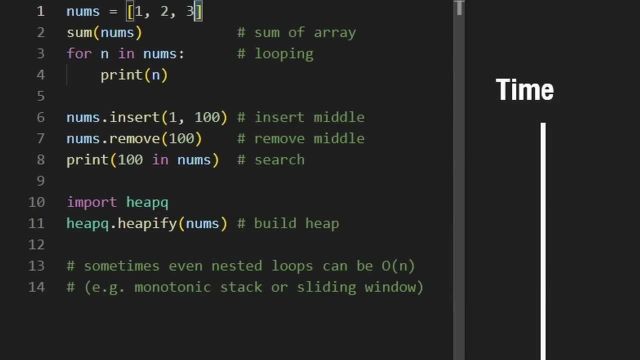 position, but we take the worst case, which is going to be big O of n, Another one that I get a lot of questions about. if you have a set of values- in this case a list of values 123, and you want to heapify them, you want to 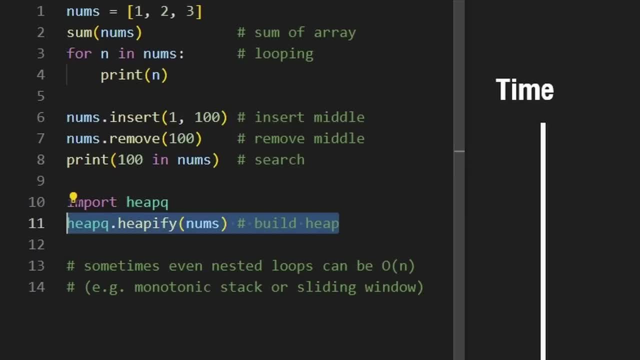 build a heap out of those elements. the heapify algorithm actually runs in big O of n time. if you don't have to individually push an element to a heap, it runs more efficiently if you can just build it from scratch. this is an end time operation, a couple more common. 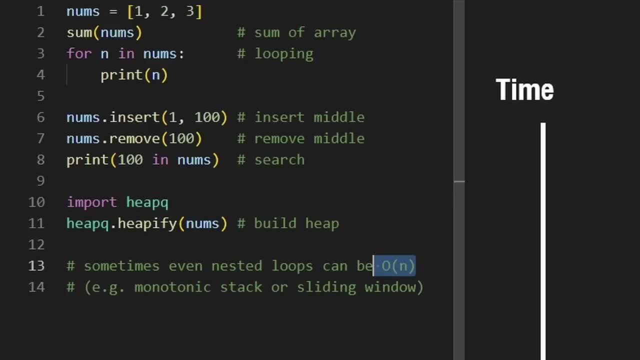 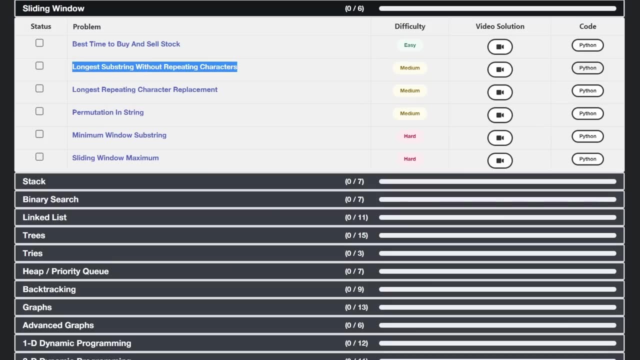 algorithms. the sliding window algorithm also runs in linear time And I'm actually going to quickly go on neatcodeio over to the sliding window section And the second problem in the list. when you take a look at the code you see that it does have nested loops, But 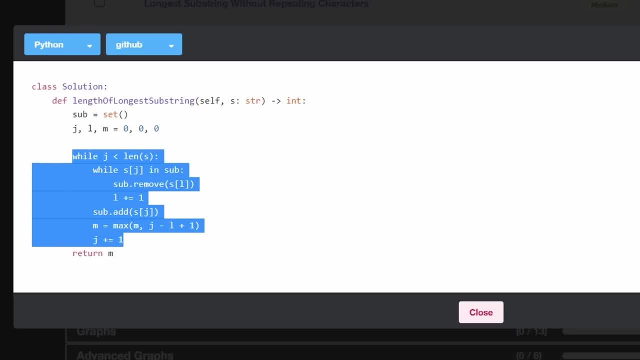 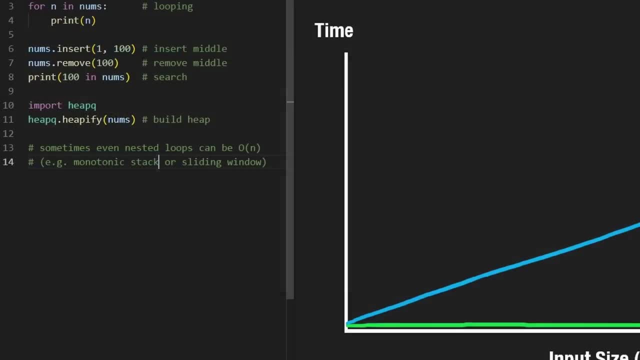 that doesn't necessarily mean the time complexity is n squared. a lot of people assume that just because you have nested loops the time complexity is n squared, But that's not always the case. The same is true for the monotonic stack algorithm. So once again going on neatcodeio to the stack. 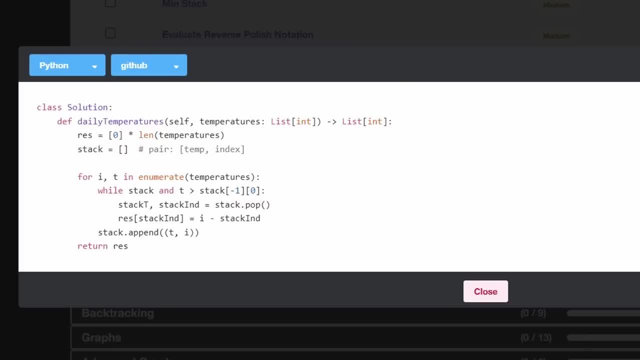 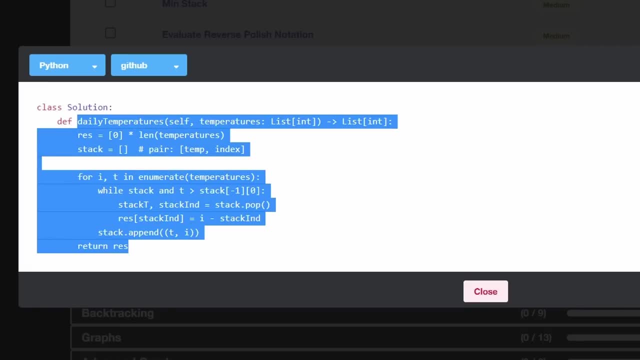 section. the daily temperatures problem is a monotonic stack problem And it also has nested loops. But this algorithm actually runs in linear time. So if you're looking for a loop, you can use it to run long term, but it's actually running in the same time. So if you want more details on 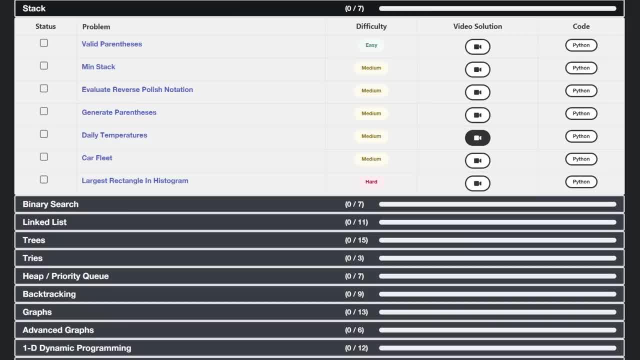 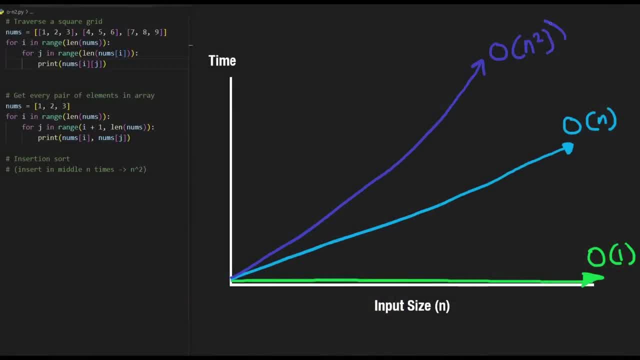 these problems, I recommend going to neatcodeio. you can check out the video explanation And I go more in depth to analyze the time complexity in each of these videos. Next, we have big O of n squared, which we kind of just talked about. when you have nested loops, the simplest case is if 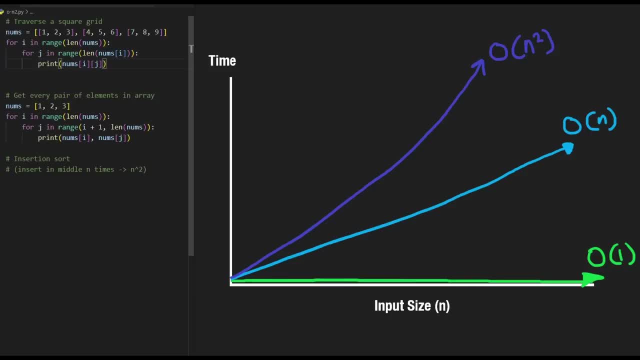 you actually had a two dimensional array and you wanted to iterate over that array, you would need nested loops to do that. So, for example, if we had a grid like this, three by three it's squared. so you know, this could be any arbitrary dimension, though n by n you want to. 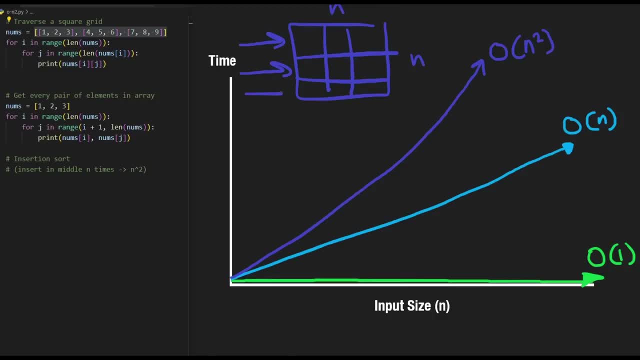 first go through every row in this grid and then, for every row, you want to go through every single position in the grid. so the outer loop is going to go through every single row and the inner loop is going to go through every position in each individual row. and what's the size of this grid? 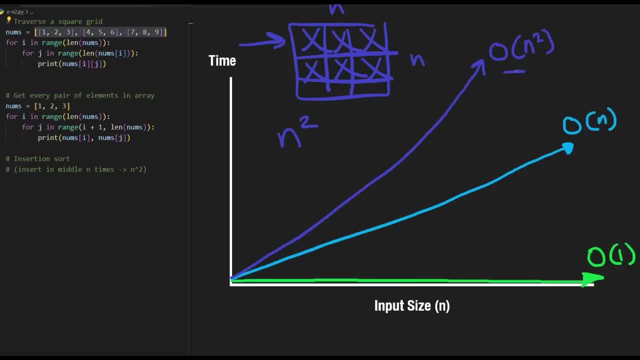 well, it's going to be n squared. that's how we get the big o time complexity. for that this is pretty simple. another case that kind of trips up some beginners is if you just have a single array and you want to iterate through it n times. so if you have an array that looks like this, of size n, you, 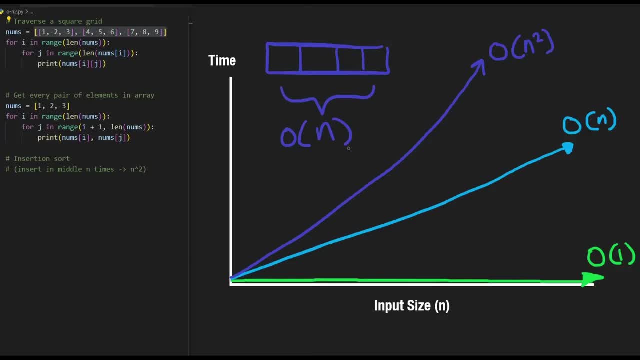 go through it once, that means the big o time complexity is going to be n. if you go through it twice, the time complexity is going to be two times n, which we know reduces to just be big o of n. but what if you iterate through this array n times? well then, the time complexity is going to 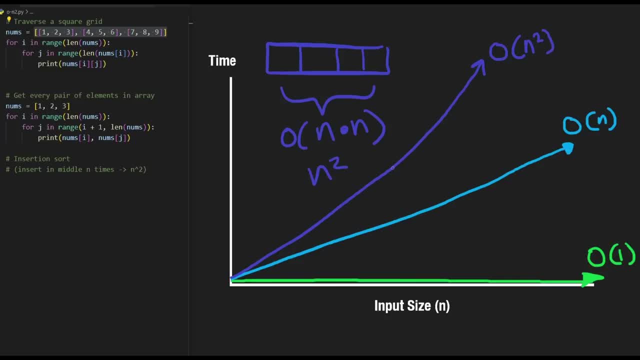 be n times n, which would be n squared. but it's actually not very common that you iterate through the entire array n times. what's more common is that you iterate through the entire array once and then you iterate through every element in the array except the first position, and then you iterate. 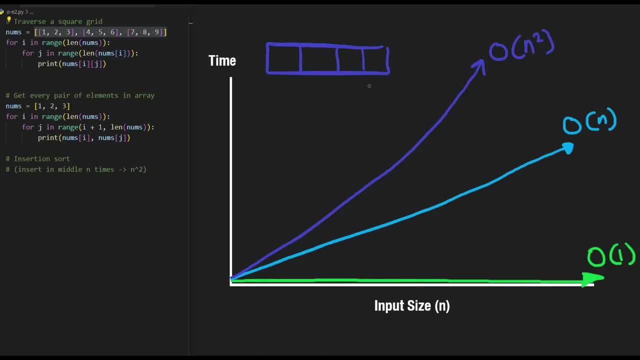 through every element except the first two positions and you keep doing this until you've just iterate through the last element. so this is a diagram of doing that. you go through four, three, two and then one. so what would be the time complexity of doing this? well, mathematically, this is actually a well-known series and it can be proven that this 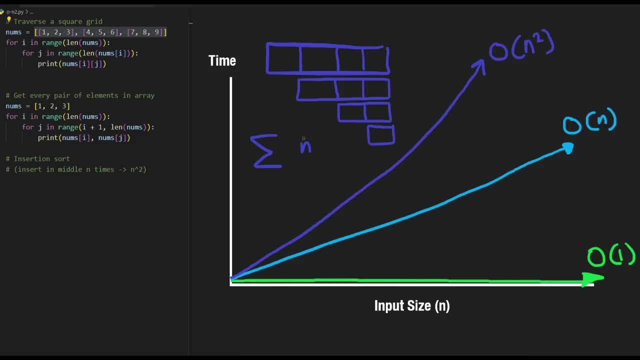 will roughly equal n squared divided by two. but if you're not smart enough or care about that math portion, an easier way to identify that would be well. here we have a square, right, we have an n by n square. now what does this portion of the square look like to you? to me, it looks like half of a. 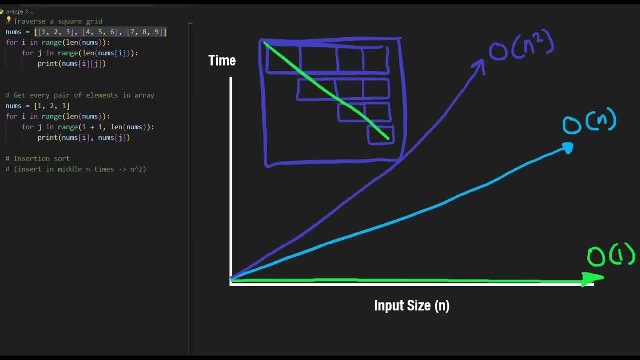 square. it basically looks like we cut this in half, so now you're probably convinced that you're going through. an array like this is going to lead us to n squared divided by two time complexity in. like I said, we don't care about constants, so this two does not matter. therefore, we say that iterating through 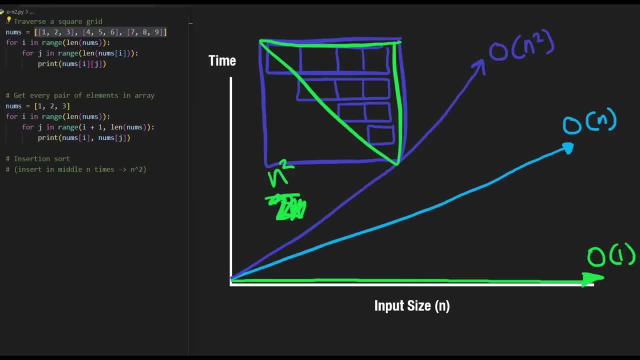 an array like this is also n squared. a lot of people kind of brush over this and I'm pretty sure most people never actually learn this or care about it. but that's okay, because you don't really need to anyway. but now you know something that probably most people don't. we also talked about 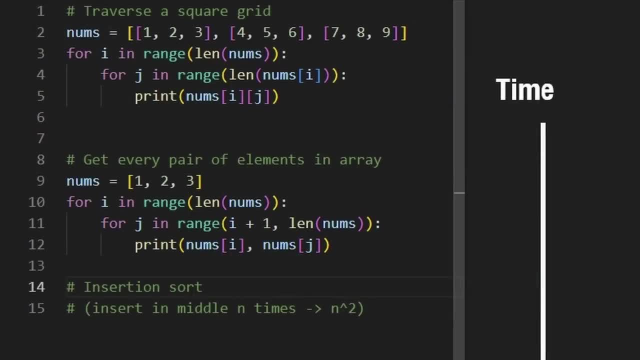 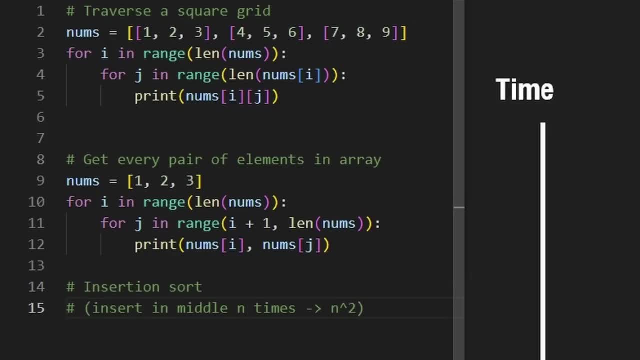 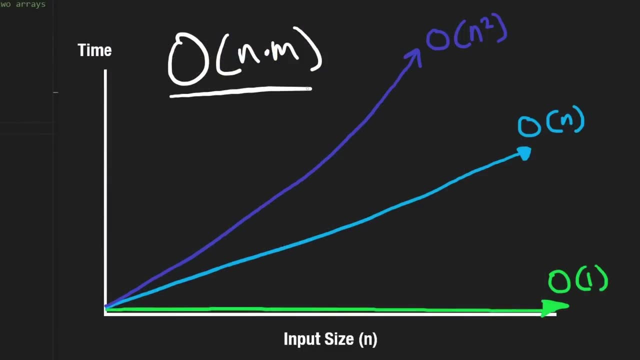 n time operation. So insertion sort, which basically inserts into the middle of an array n times, is going to have n squared time complexity as well. Another one that's pretty similar to n squared, so I won't actually draw this one out on the grid, but n times m This. 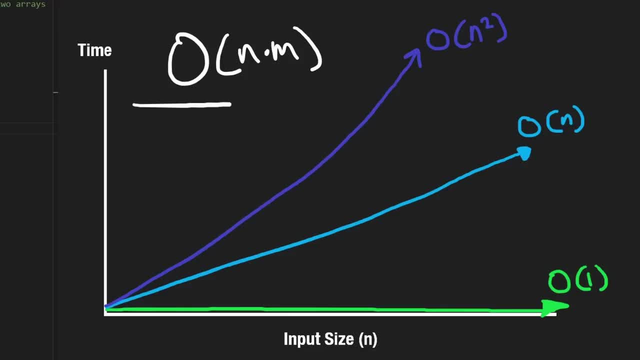 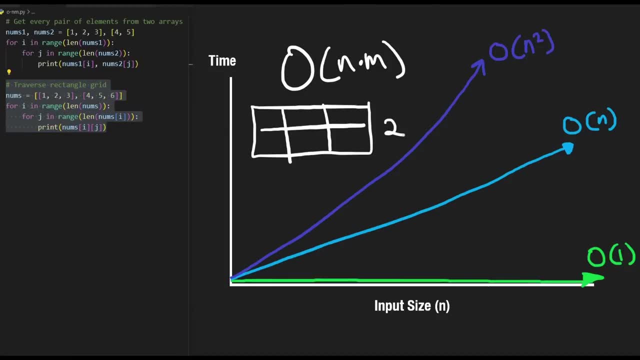 could mean a two-dimensional matrix, that's not necessarily a square. So in our example on the left over here, we could have some rectangular array that looks like this, where we have two rows and we have three columns. So in this case n might be the number of rows, where m might be. 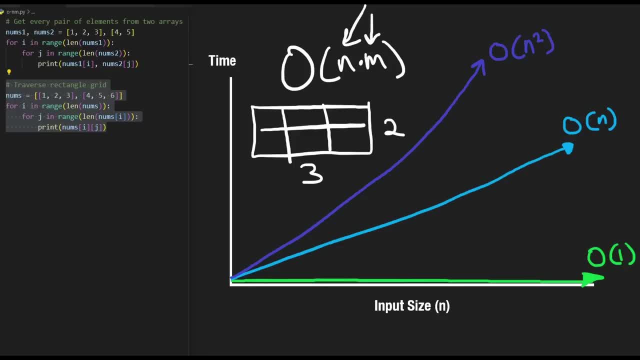 the number of columns. We actually have two variables this time, which is perfectly valid in big O notation. Now, if we can have n squared, why stop there? We can also go up to n cubed, and we could actually go higher and higher to n, to the power of four, to the power of five. 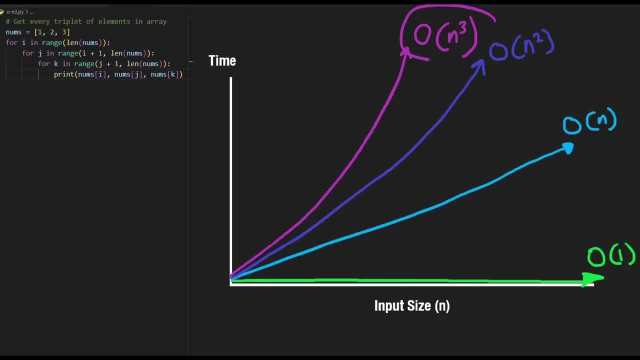 et cetera, et cetera, but I won't do that. It's pretty uncommon to even have n cubed, actually for most problems, but this is usually the highest that we get to. Usually you don't have algorithms that go up to n, to the power of four, but it's possible. 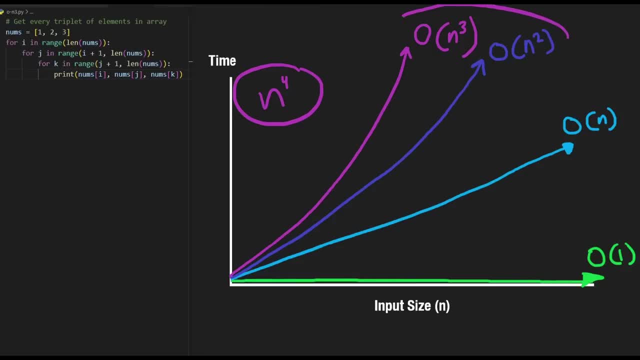 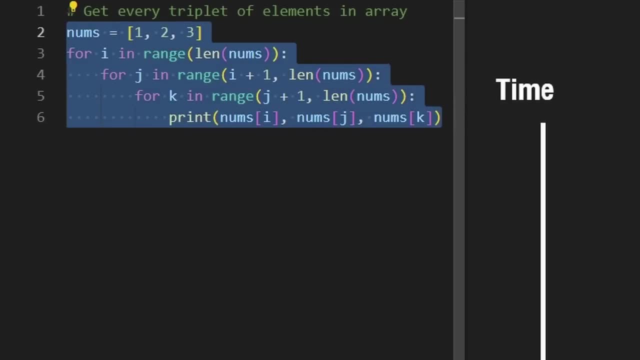 and I think you would be able to identify that case. if you're able to identify these as well, Of course we could have some kind of three-dimensional data structure. More commonly, though, you'll just have a single array, and you'll want to get every unique triplet from that. 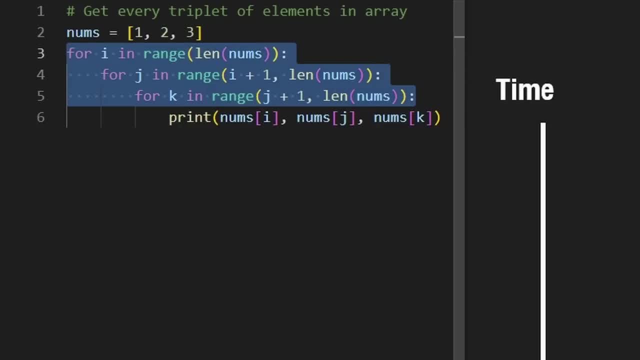 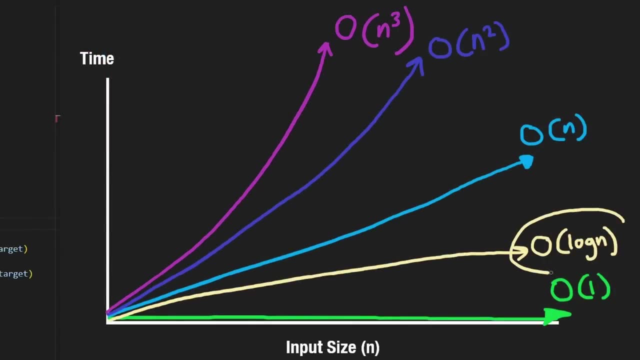 array, for example. So in this case we would need three nested loops to iterate through every single triplet from this input array. Now let's move on to some of the more complicated ones, like log n. This is where we get more math involved and I bet you most people don't know how to analyze log n. 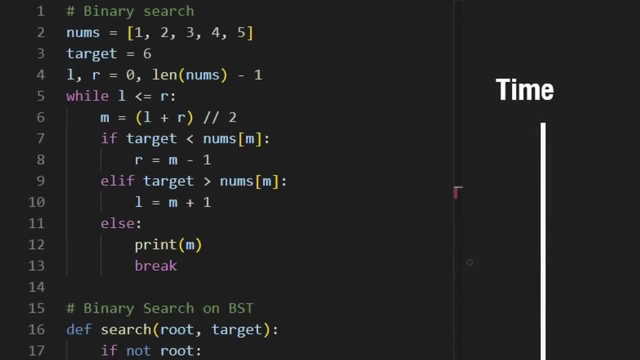 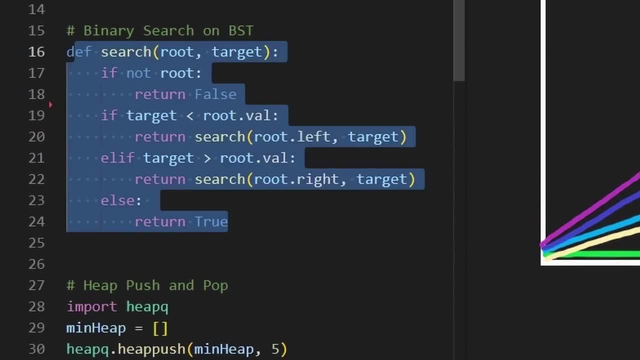 time complexity. They kind of just memorize it, because usually log n is applied to binary search, for example on an array, or you could run binary search on a binary search tree. These are the two most common algorithms, but there's also pushing and popping from a heap, which is another common. 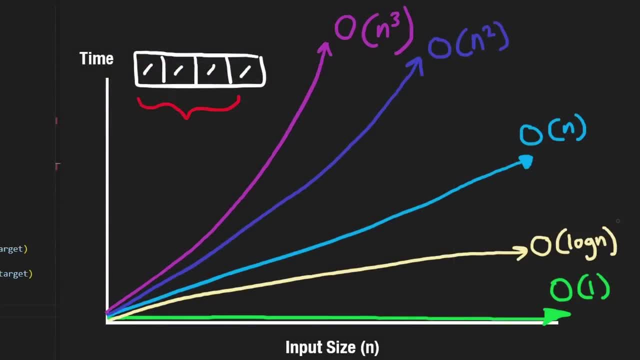 one On an array. the reason binary search runs in log n time is because on every iteration of the loop we allow the binary search to run on a binary search tree and that's the reason why we don't have eliminate half of the elements from like consideration. we don't need to search this. 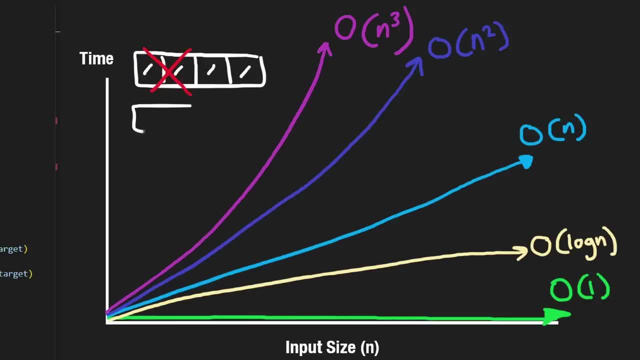 half of elements, for example. so then we'd be left with two elements and we could keep cutting this array basically in half until we have nothing remaining. that's when we would have completed our binary search. so the question is: given an array of size n, how many times can you cut the? 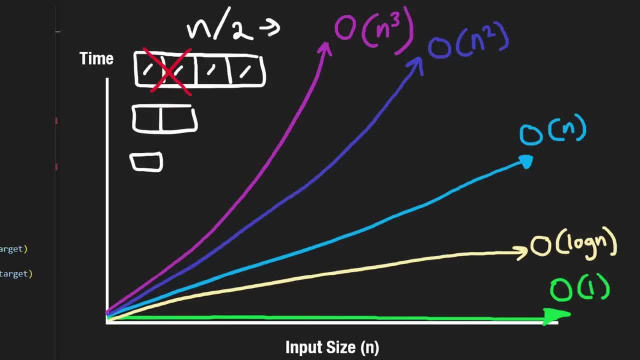 value n by two. how many times can you divide it by two until it equals one? well, another way of talking about this would be: how many times can you take the value one and multiply it by two until it's equal to n, aka two to the power of what x, in this case, is equal to n? how do we solve this? 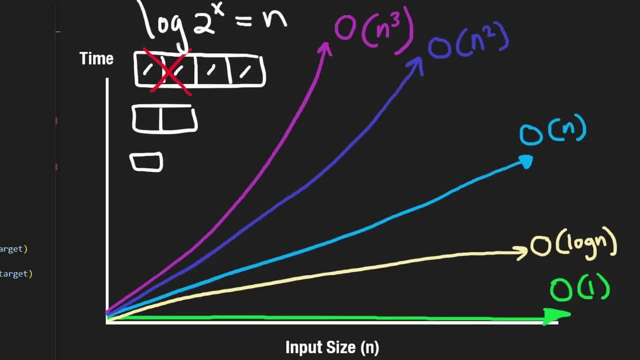 mathematically. well, by definition, that's what log actually is. we take the log of both sides and then we realize that x is equal to log n. so therefore, the number of times you can take an array like this and divide it by two is equal to log n. 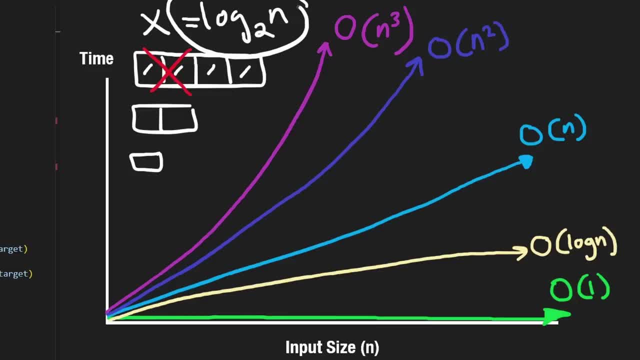 in this case, the base of our logarithm is going to be two, so that's where this comes from, and the idea is the same when we're talking about binary search trees, at least if your bst is balanced, because as we search it, we're either going to go to the left or to the right looking for some target. 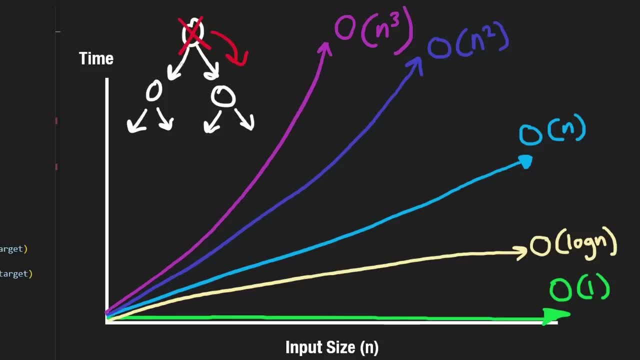 value. so if we end up going to the right, that means we eliminated the entire left half of the tree from consideration, and we do this recursively. so we start with a tree of size n and we basically remove half of the elements from consideration until we find the target that we're looking for. that's why this is also a log n time algorithm. 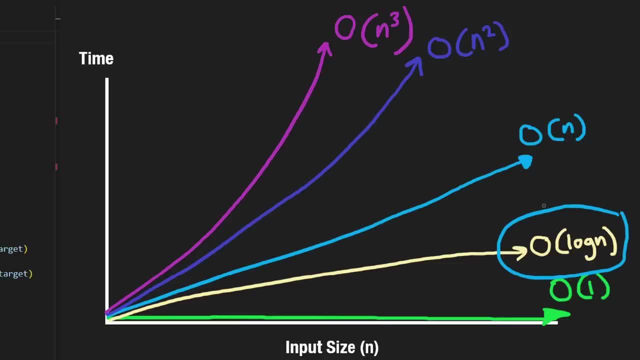 so log n grows pretty slowly. you can't tell from this chart. but actually for really really large input sizes log n is practically a flat line like the difference between log n and big o of n is massive. i think log base 2 of 4 billion would be something like 32. so even with an input of 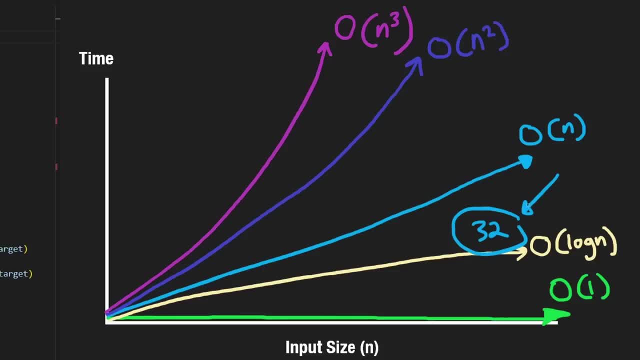 billions, we get a very small two digit number. now we also have n multiplied by log n and this is actually only marginally less efficient than big o of n. it's a lot more efficient than n squared, just like how log n is much more efficient than big o of n. the most common algorithms for n log n are sorting, for example, merge, sort and. 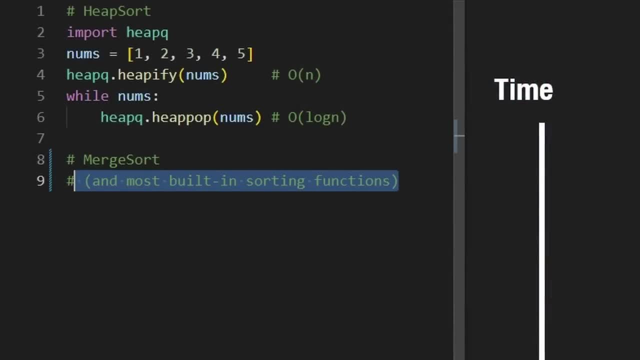 we usually assume that most built-in sorting functions are n log n. so if you need to run the built-in function in a coding interview, you can basically assume that it's an n log n algorithm. heap sort has the same runtime and this kind of illustrates how we can get a runtime like: 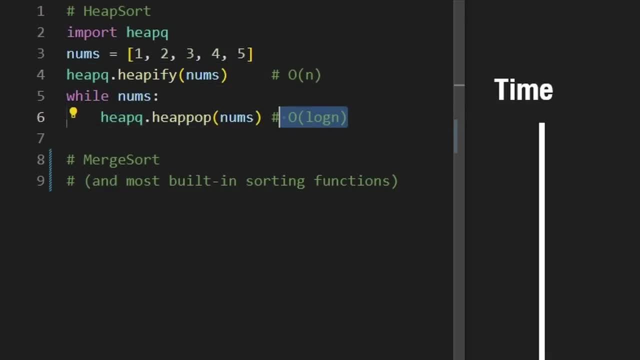 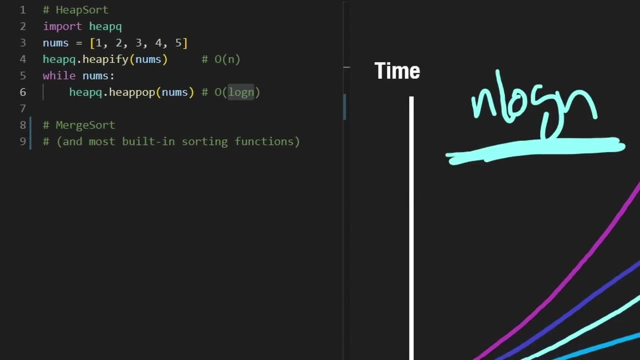 this: we know that popping from a heap is a log n time operation, and if we have a heap, you know, of size n and we have to pop from that heap while that heap is non-empty, then we end up doing n operations which take log n each. therefore, we get n log n as the total result. now, in this example, 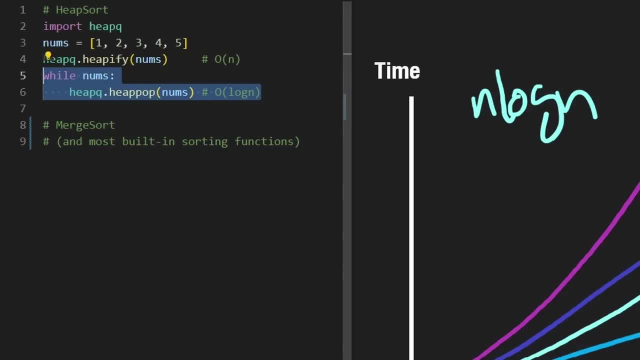 before we started running the heap sort algorithm, we actually had to build the heap, so this took big o of n times. so actually the overall runtime was n plus n log n. should we draw that on our chart? well, with big o notation, we only care about the larger term. if we have a term like this, which 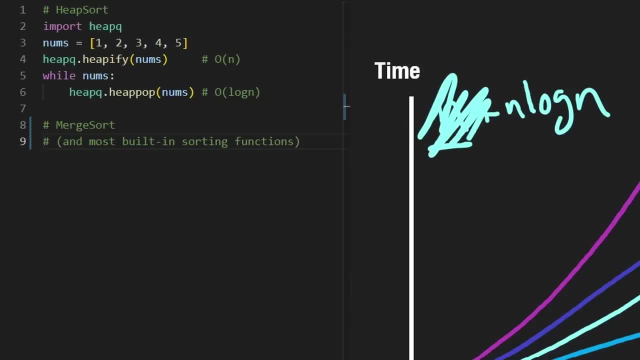 is strictly larger than this term. we don't care about the smaller term, but we could have a time complexity where we have m plus n, log n and in this case, since m is a different variable from any of the variables we have here, we don't know that this is a. 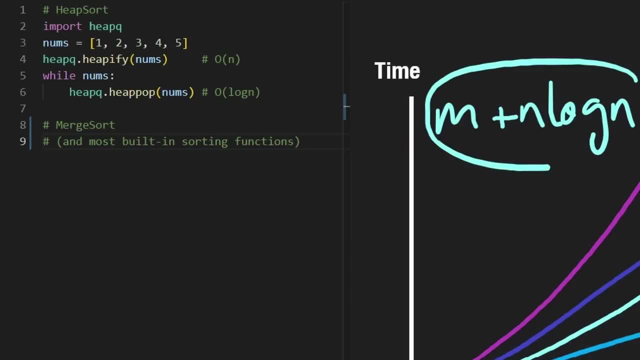 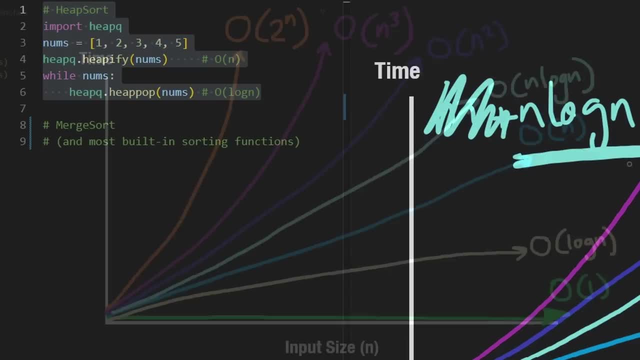 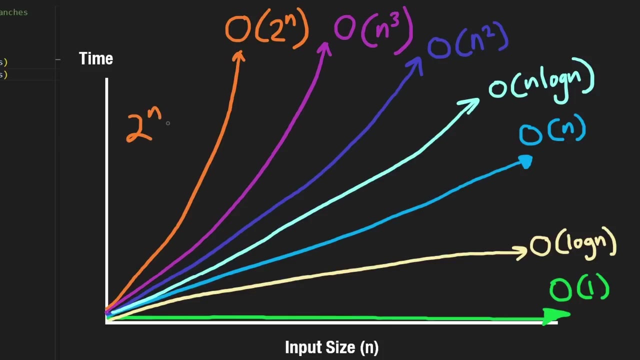 smaller than this one. so we have to include both of these in the big o time complexity. but we don't have that in this case, so we reduce the time complexity to just be n log n. now let's get into some of the non-polynomial runtimes which, starting with the most common, is 2 to the power of n and. 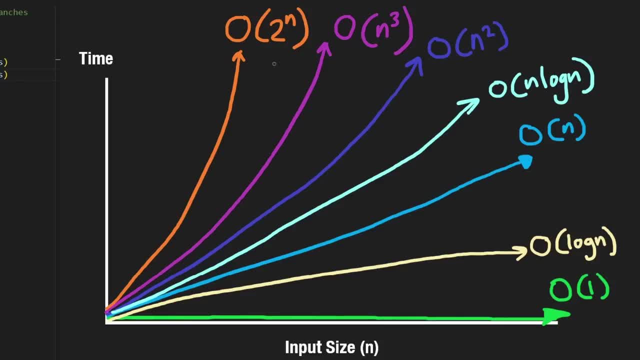 this is the part where i could start going on a nerd tangent and talking about how this equation is actually just a reflection of the log n over. you know this axis, but i'm pretty sure nobody cares about that, so i will just go ahead and do that, and i'm going to go ahead and do that, and i'm going to. 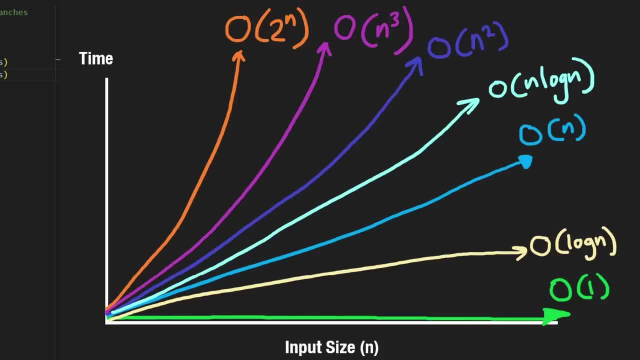 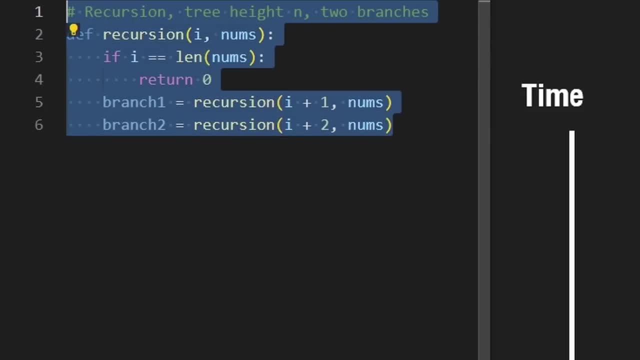 get into it, but feel free to comment if you're interested in the math stuff. it's most common to have a runtime like this when you're talking about recursion. so this is an example of two branch recursion, where our recursive tree will have a height of n, but we'll have two branches every. 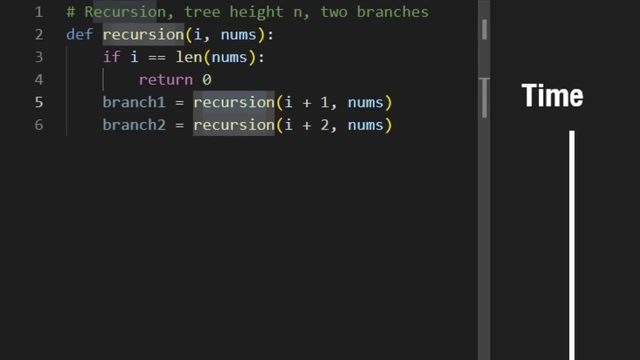 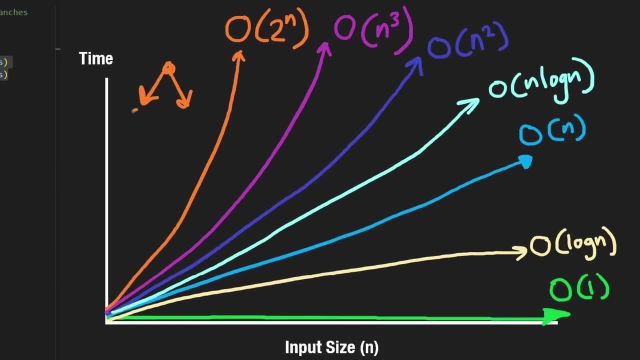 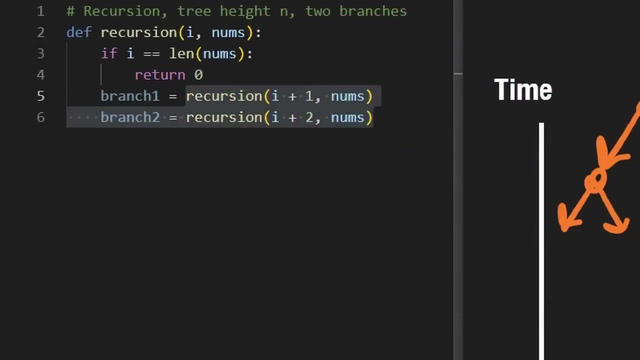 time. so this is recursively calling some recursive function. it's not really doing anything. but here you can see we have two branches of recursion. visually it would look something like this, you know, similar to a binary tree, but in this case the height of this tree would be measured in terms of n. so, for example, if we were given some input array of 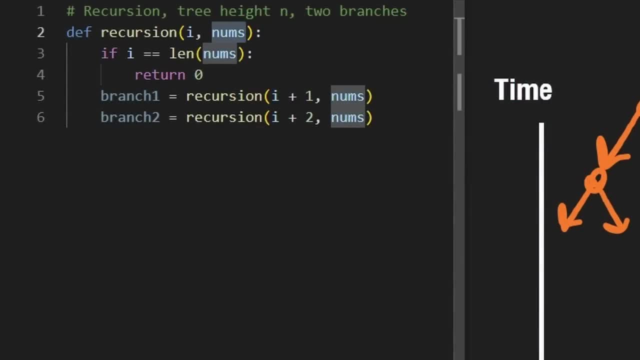 size n and we wanted to get all possible combinations. that would be one example of two to the power of n runtime. so, for example, computing the fibonacci sequence recursively is a pretty common example. or combinations. now, if we can have two to the power of n, can't we have? 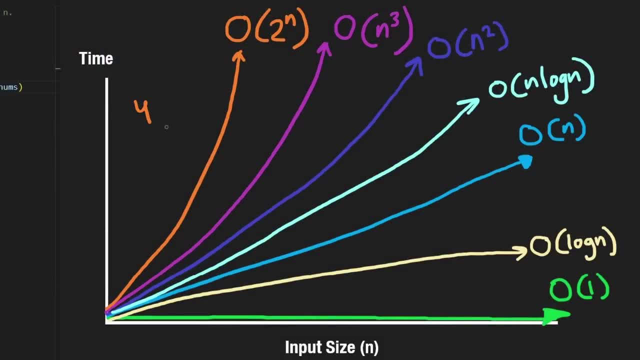 three to the power of n, and what about four to the power of n? yeah, you can have pretty much any constant. let's call it c raised to a power of n. so we can have two to the power of n and we can have three to the power of n. now, i'm not going to draw those out, but with a bigger base value we will. 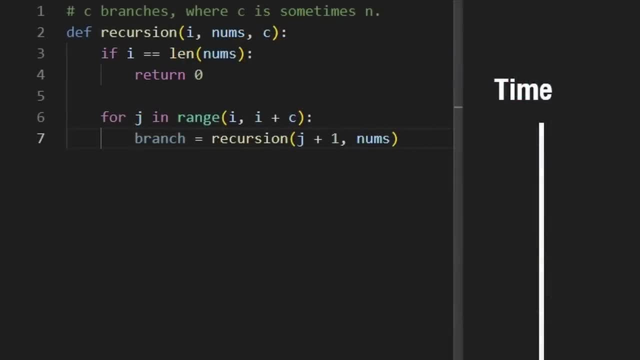 have, you know, increased runtime complexity. so an example of that would be pretty similar to our previous recursive example, but in this case, instead of having two branches, we have an arbitrary number of branches, so we use a loop to do that. so in this case, our constant c is going to tell us how many. 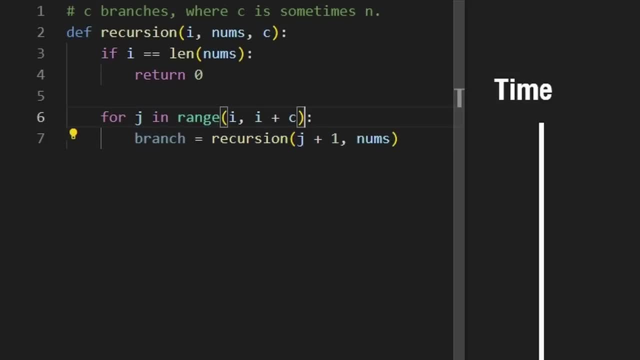 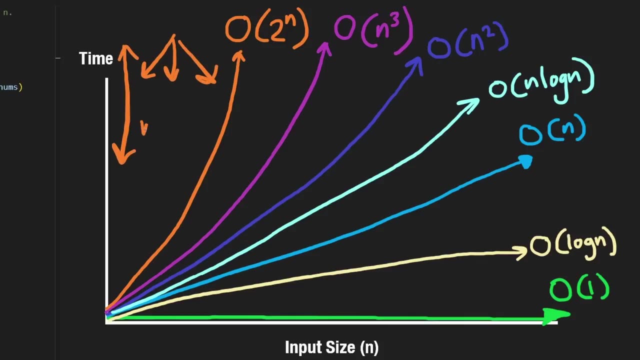 times we need to loop and make a recursive path. so in this case, if c was 3, we'd have a decision tree with three branches and the height of the tree would continue to be n. so we would end up with a time complexity of three to the power of n. now how am i getting that time complexity from a decision tree? well, 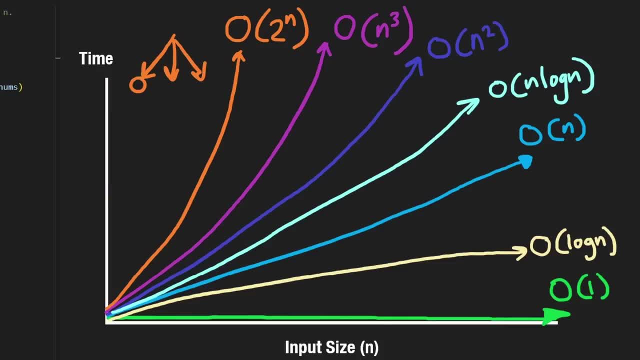 think about it this way: if we have three- uh, you know- branches on the first level, we have three values here. now for each of those, we're gonna have three more branches, and then for each of those we're gonna have three more branches. we're basically gonna keep doing this. 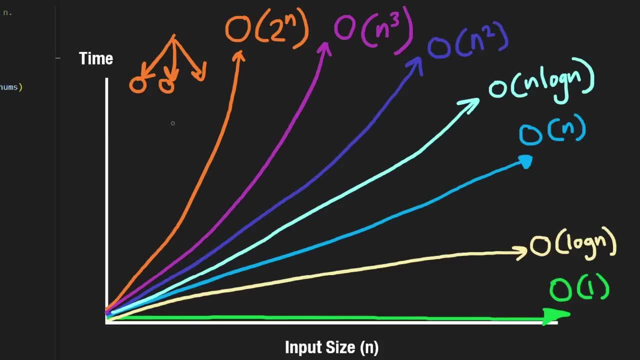 until we reach the entire height of the tree, which in this case is n. So we're basically going to have a number, our base value, three, multiplied by three, and just keep multiplying it until we have n of these. Therefore, we get three to the power of n. Now a pretty rare runtime. complexity is the square root of n. 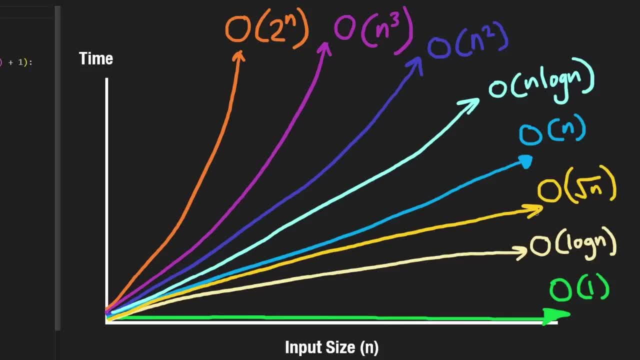 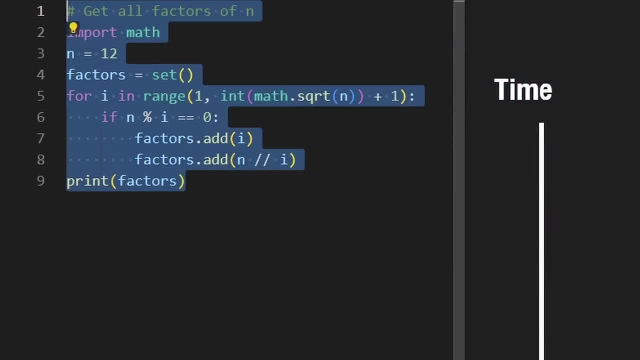 you rarely see this, but I still think it's worth mentioning. you will rarely ever see this in a coding interview, But I think it's still worth mentioning. The only example I think I've ever needed this for is getting all the factors of some value. So, for example, if we're given a value, 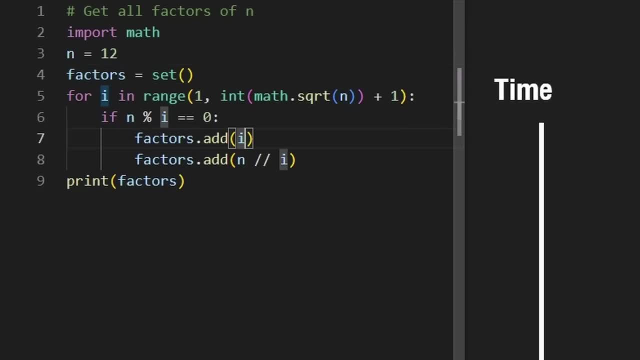 n and we want to get all the factors of it. we will go through every value between one and the square root of n and check if any of those values is a factor of n And since this could possibly produce some duplicate factors, we add those factors to a hash set which we know is a constant. 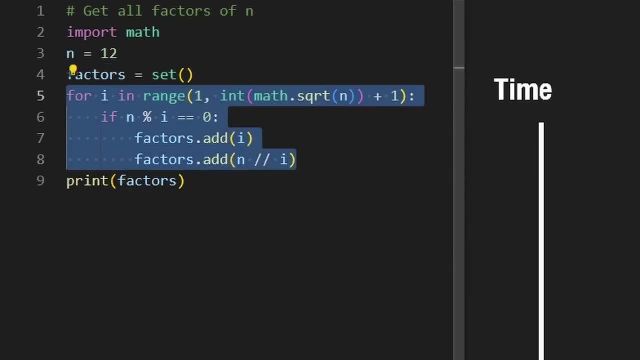 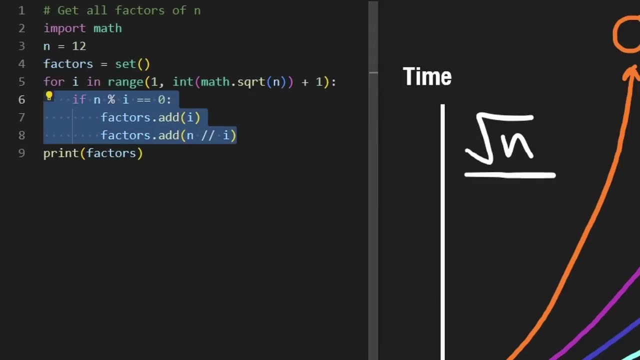 time operation. So the number of times this loop is going to execute is, of course, going to be the square root of n. Now I won't go super in depth on why this algorithm works. If you want to know, feel free to ask in the comments. It's really more of a math problem than a coding problem. 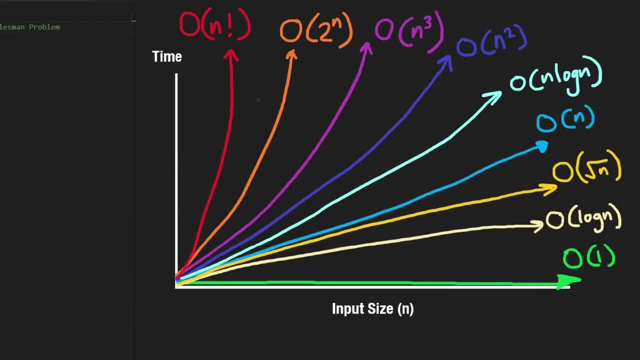 And lastly, we have n factorial, which is a math equation, which basically means: you know, if we had five factorial, that is five times four times three times two times one. So basically it ends up being a very big number. we say that this is bigger than two to the power of n. 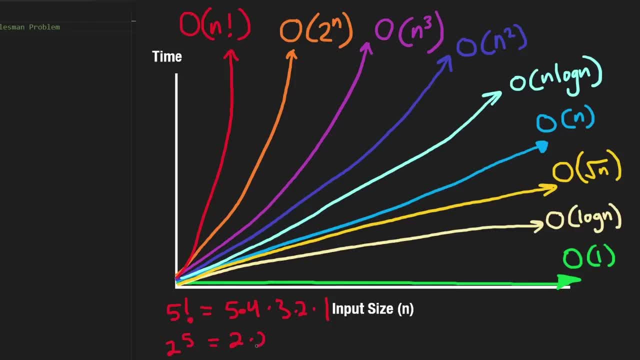 because two to the power of five is a factor of n, So we're going to have n. factorial in this case would be two times, two times two, five times, And you can see that just by looking at these two cents factorial has the potential for having larger terms than just some constant. 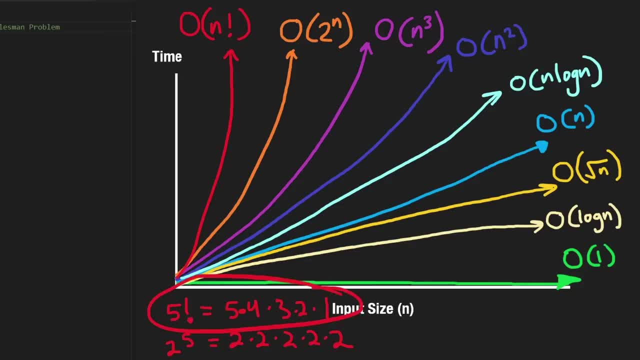 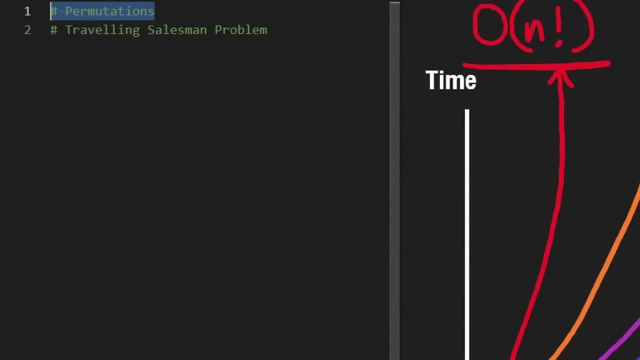 value two or three or four, that this is going to grow much quicker than this one. Now, n factorial is pretty rare. It mainly comes up for permutations and sometimes in graph problems, for example the traveling salesman problem. But I think you don't have to focus too much on n factorial. 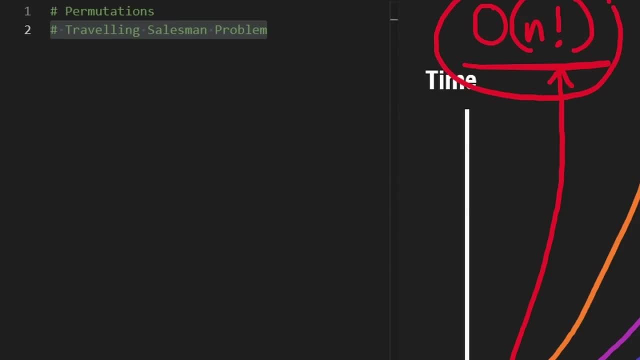 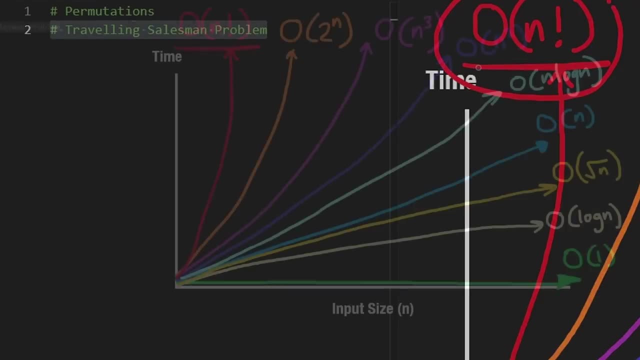 you mainly have to know that it's very inefficient. So if your solution is n factorial, most likely you don't have the optimal solution, But sometimes n factorial is the best you can do in a real interview. I don't think it would matter too much. if you can, you know precisely tell. 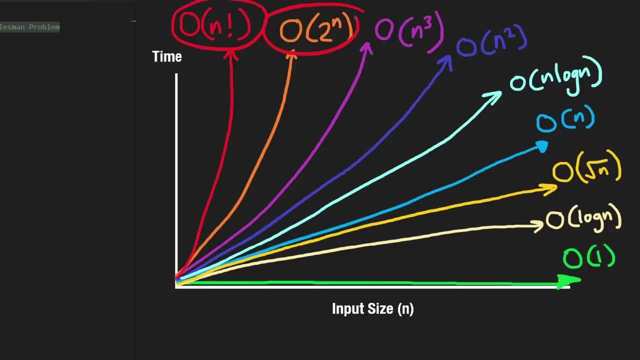 is your algorithm n factorial or is it exponential to the power of n? it wouldn't matter a lot. And also knowing the exact difference. for example, the square root of n is actually growing quicker than log n. you could kind of figure that out just by doing some. 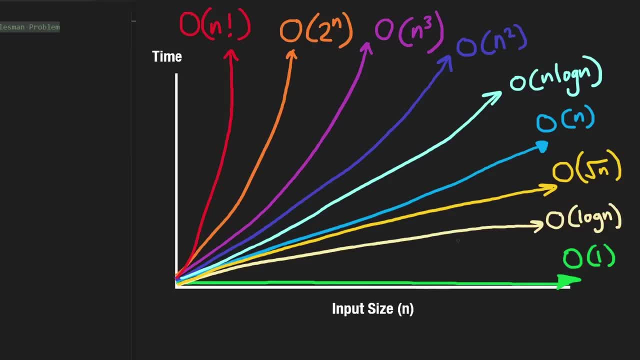 math in your head. Like I said, the log of 4 billion is going to be something like 32, whereas the square root of 4 billion is still going to be a very large number. But this is mainly to give you a high level overview of how these time complexities relate to each other. 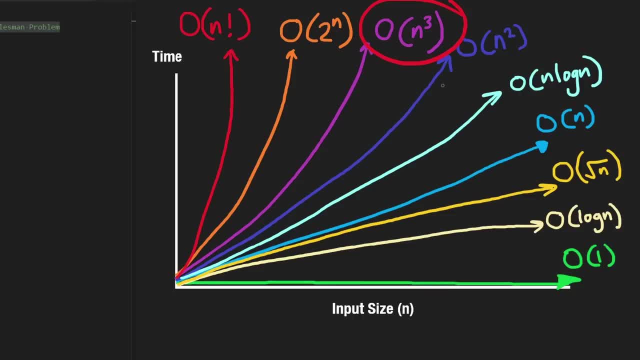 because that's what's important. you need to be able to know how efficient your algorithm is. if you see your algorithm is factorial or exponential or even n cubed, you know it's not super efficient. you want your algorithms to be on the right side of. 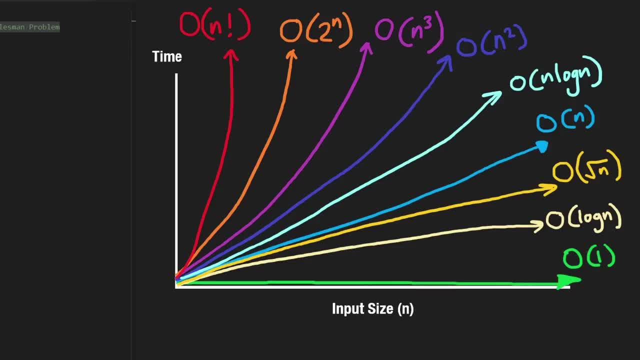 this chart, though sometimes it's not possible. If you found this video helpful, please like and subscribe. it really supports the channel a lot. If you're preparing for coding interviews, check out neatcodeio. it has a ton of free resources. you can also get 10% off lifetime. 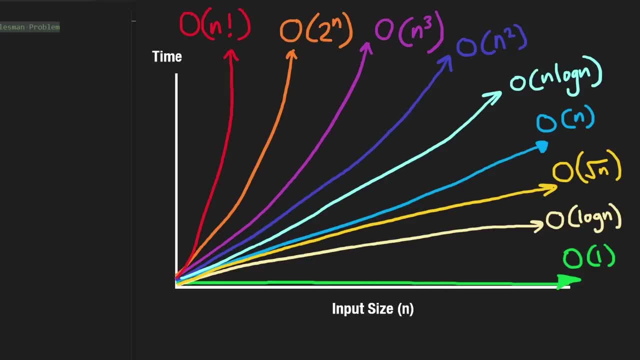 access using code neat. Thanks for watching and hopefully I'll see you pretty soon.